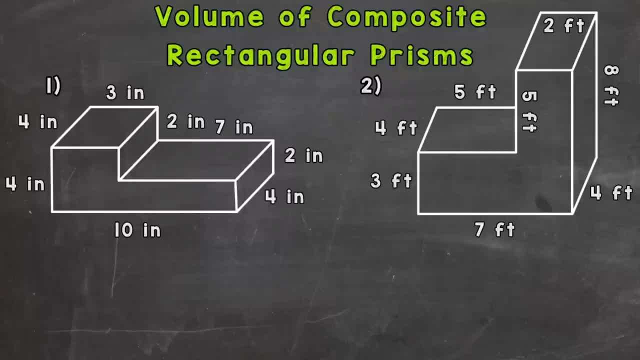 this down Now. you might remember, or maybe you forgot, and this is a quick refresher, but the formula for volume that we are going to use is length times width times height. And remember, volume is the amount of space a three-dimensional object takes up And, as you can see, these aren't. 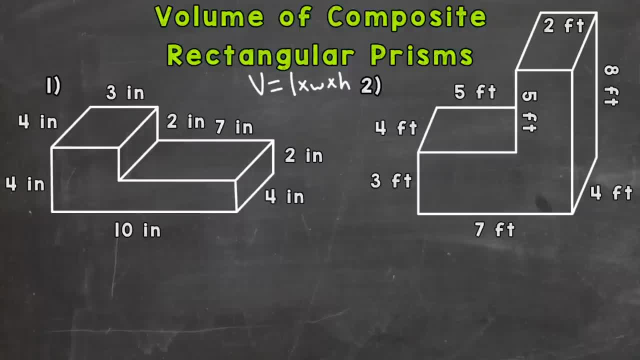 just plain old rectangular prisms. They're a little more complex, so it takes a couple extra steps, but the foundation of finding the volume is still going to be that formula. So let's jump right into number one here And when we have composite rectangular prisms, the first 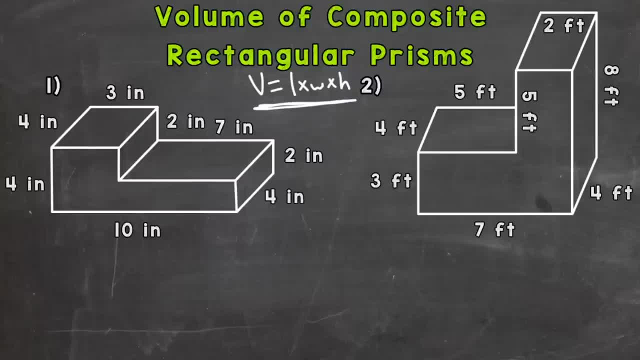 thing we want to do is cut that figure into two separate rectangular prisms. So I'm going to draw a line here that's going to separate this into a left and right rectangular prism. I'm going to call the left hand one A and the right hand one A. So I'm going to call the left hand one A and the 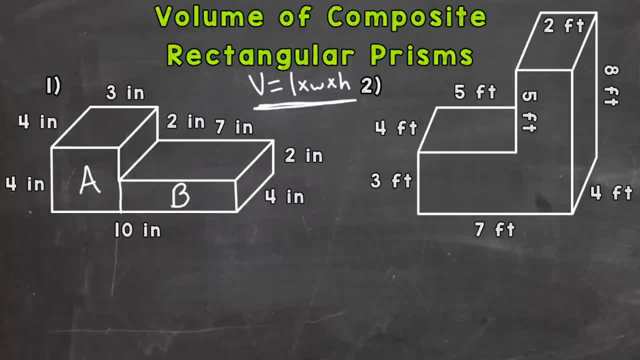 right hand, one B Again. I cut the complex or composite figure into two rectangular prisms. Now what we're going to do is find the volume of A, the volume of B and add those together And that's going to give us the volume of the composite rectangular prism. So let's do A first. So I'm 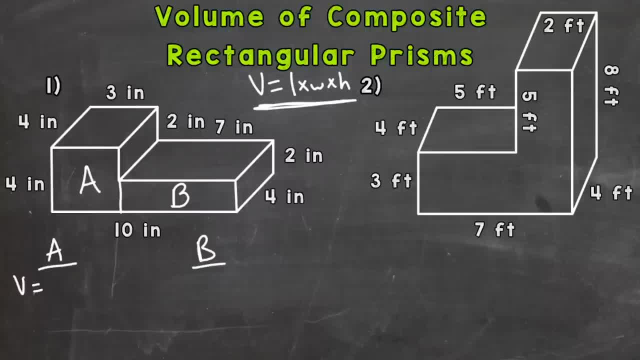 going to put our A and B together, And then I'm going to put the volume of A and B together, And then let's write out our formula for each And once we get to this part, it's about picking out the correct lengths, widths and heights for A and B. So again, let's do A first. So we need. 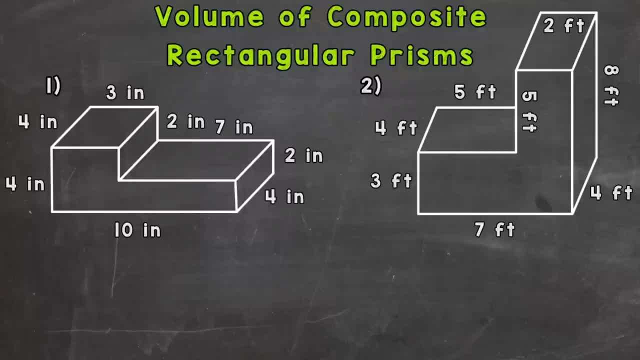 this down Now. you might remember, or maybe you forgot, and this is a quick refresher, but the formula for volume that we are going to use is length times width times height. And remember, volume is the amount of space a three-dimensional object takes up And, as you can see, these aren't. 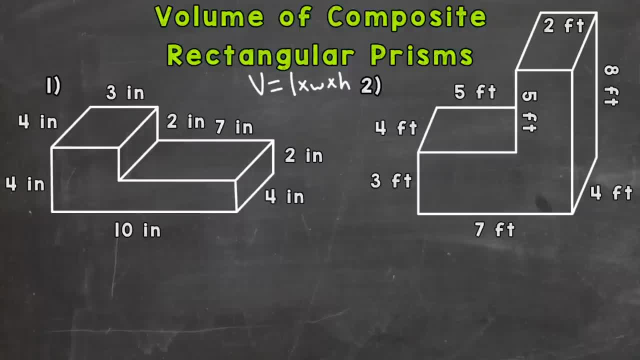 just plain old rectangular prisms. They're a little more complex, so it takes a couple extra steps, but the foundation of finding the volume is still going to be that formula. So let's jump right into number one here And when we have composite rectangular prisms, the first 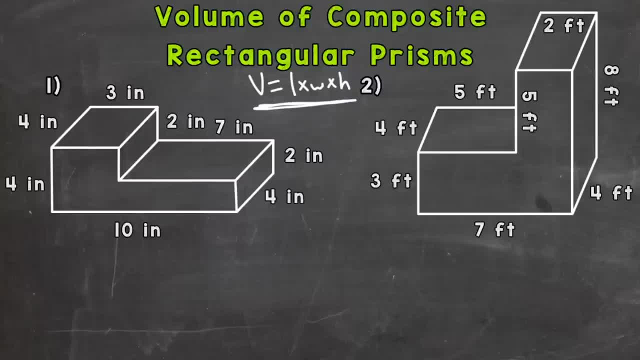 thing we want to do is cut that figure into two separate rectangular prisms. So I'm going to draw a line here that's going to separate this into a left and right rectangular prism. I'm going to call the left hand one A and the right hand one A. So I'm going to call the left hand one A and the 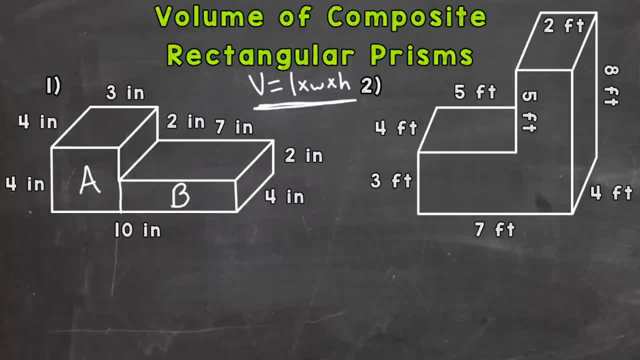 right hand, one B Again. I cut the complex or composite figure into two rectangular prisms. Now what we're going to do is find the volume of A, the volume of B and add those together And that's going to give us the volume of the composite rectangular prism. So let's do A first. So I'm 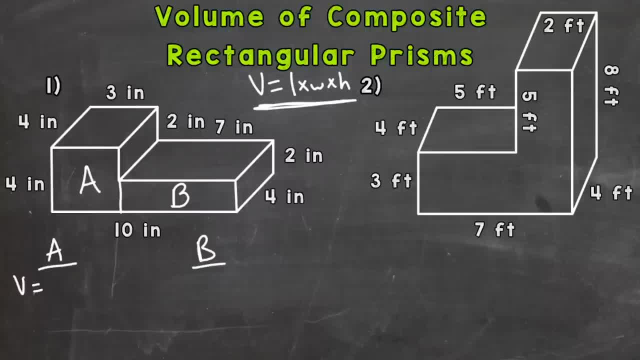 going to put our A and B together, And then I'm going to put the volume of A and B together, And then let's write out our formula for each And once we get to this part, it's about picking out the correct lengths, widths and heights for A and B. So again, let's do A first. So we need. 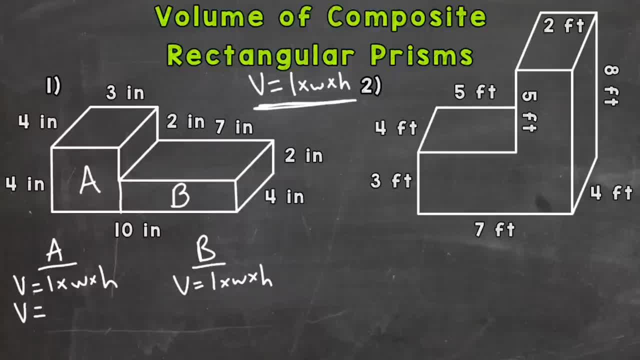 the length- And I consider the length- how far back that rectangular prism goes. So we're going to want to see how far back- And that's going to be four inches times how wide is A. So A goes from there to there. So we're not going to use that 10 inches. 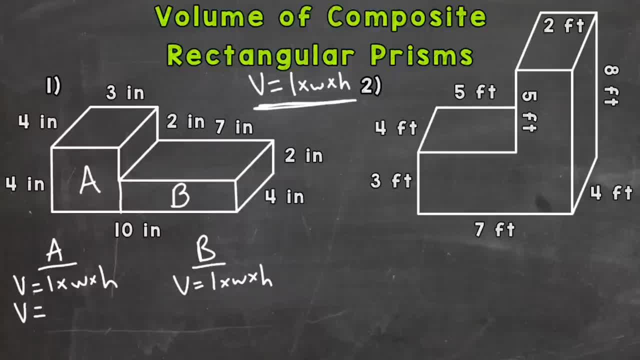 the length- And I consider the length- how far back that rectangular prism goes. So we're going to want to see how far back- And that's going to be four inches times how wide is A. So A goes from there to there. So we're not going to use that 10 inches. 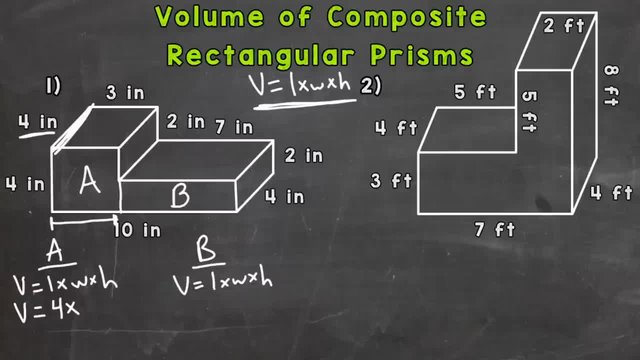 That's a common mistake: using incorrect measurements. That 10 inches goes all the way across. We just want right here. So we're going to like put our A and B together, And then we're going to have to look around this rectangular prism in order to find the correct number And 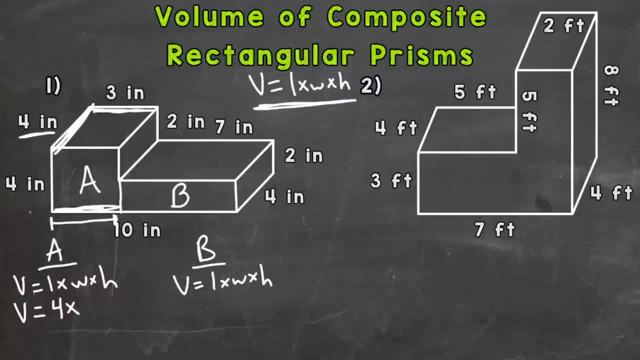 if you look up top, we have a three inches that matches with the width, So we're going to plug in that three, And next is the height, And we could look here at this four inches for that. So we need to do four times three times four. 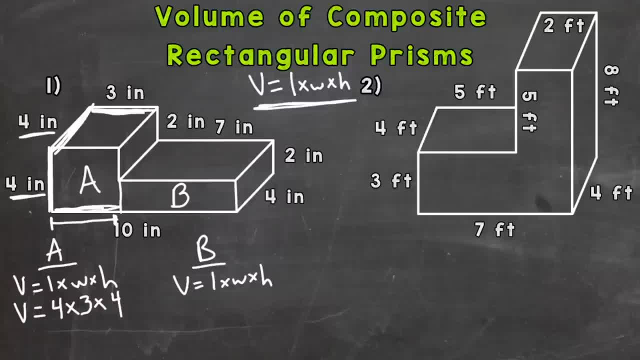 In order to calculate the volume of part A, Four times three is 12.. Times four is 48. And these are cubic inches. Now we're halfway done with the problem, because that is the volume of just A. Now we need to do B. So the length, How far back? Well, four inches. 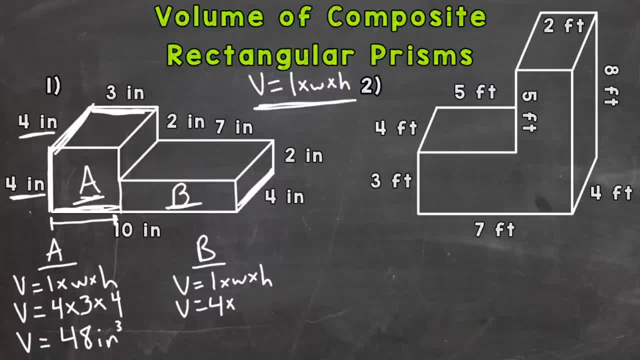 Don't use that 10 inches because we want the sum last one here, Just the size of B. So this is the width. thickness is going to be this one Times pyramid. this is knows under the 0.. So that's to where the Hebrew is in the preserve area And the middle. So this is the 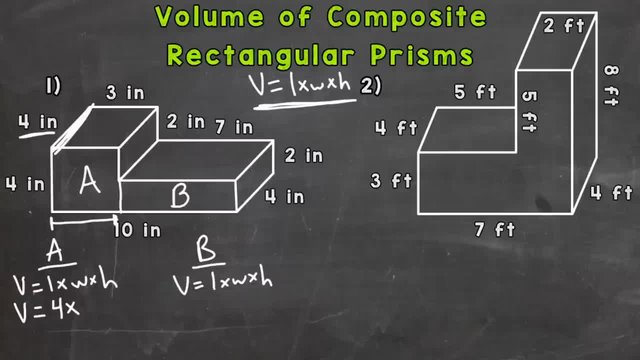 That's a common mistake: using incorrect measurements. That 10 inches goes all the way across. We just want right here. So we're going to like put our A and B together, And then we're going to have to look around this rectangular prism in order to find the correct number And 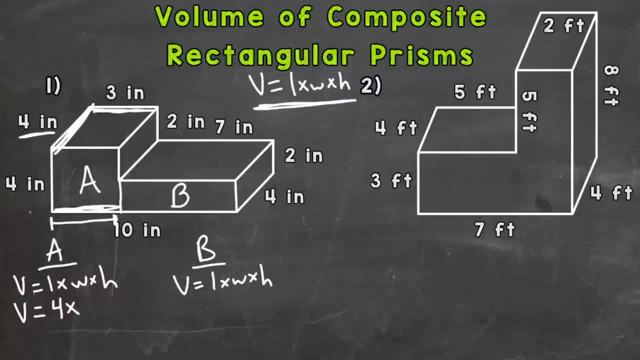 if you look up top, we have a three inches that matches with the width, So we're going to plug in that three, And next is the height, And we could look here at this four inches for that. So we need to do four times three times four. 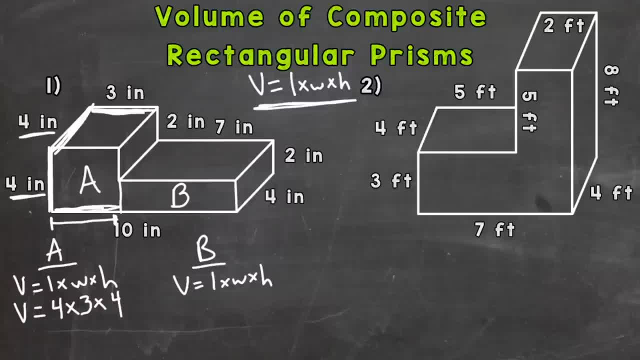 In order to calculate the volume of part A, Four times three is 12.. Times four is 48. And these are cubic inches. Now we're halfway done with the problem, because that is the volume of just A. Now we need to do B. So the length, How far back? Well, four inches. 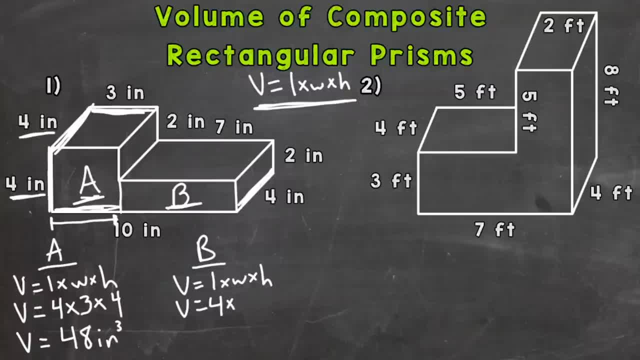 So what's the space right here? again, We know B goes to straight forward. So what's the area over here exactly? Oh, it's the area. What is it? It's a two- Ingredient: rainbow, A symbol, toan, Java, A symbol. to then The width right here is 12.. 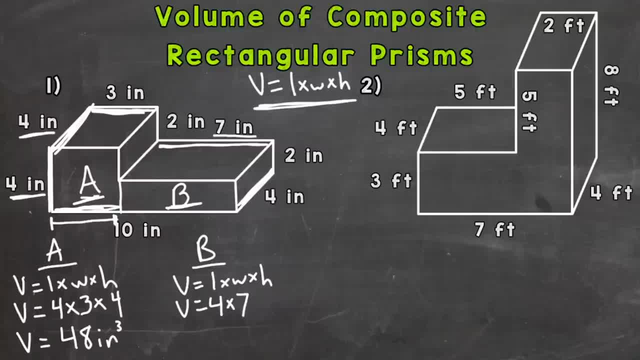 width of the pyramid. Now, the再來ичегоi is just the size of the square And it would be two times The width eg d don't ulessly a tenn. tenn goes all the way acost. that includes, Maybe you want a and b. we just wa nt the w if hre, which is going. 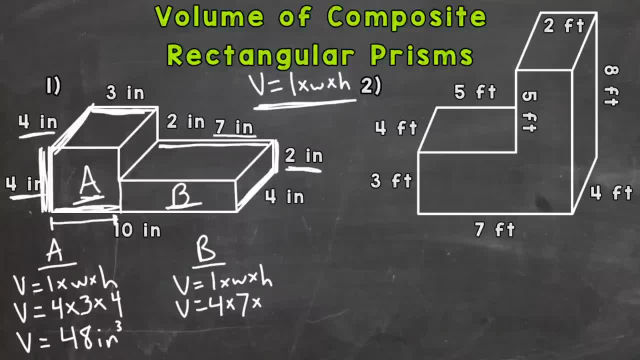 to be 7 inches. We just want the width here, wich is going to be seven inches, And then the haigh And then the height. I Well b isn't this full four inches that we used for a little bit shorter so lot. And this 2 inches is our height for B. 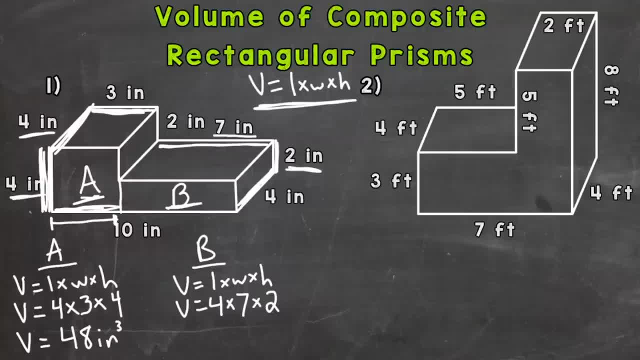 So 4 times 7 is 28.. Times 2 is 56. And that's cubic inches. So now to wrap up the problem, I'm going to go to the top left of the screen where I have some room. here We need to do B, which is 56,, plus A- 48, to get the total volume. 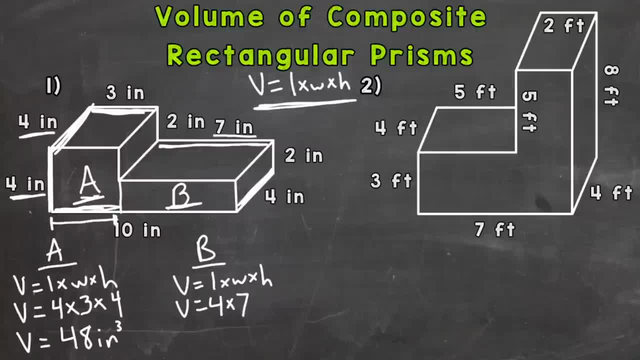 Again, don't use that 10.. That 10 goes all the way across. That includes A and B. We just want the width here, which is going to be seven inches, And then the height. Well, b isn't this full four inches that we used for A. 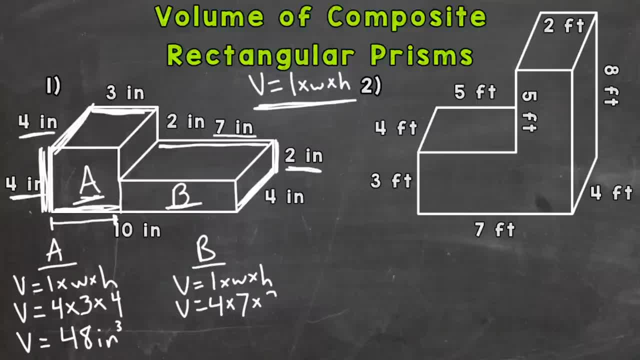 It's a little bit shorter. So let's look back here and this two inches is what's gonna be here. inches is our height for B. so 4 times 7 is 28, times 2 is 56 and that's cubic inches. so now to wrap up the problem, I'm going to go to the top left of the. 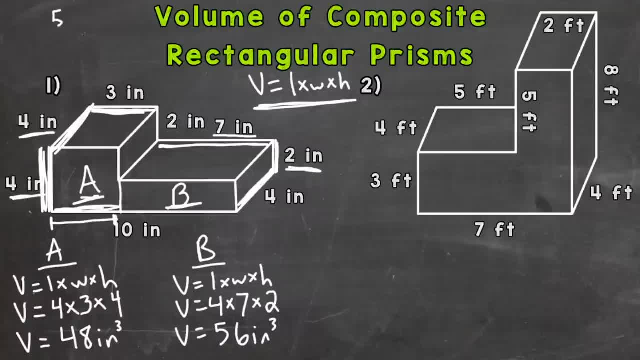 screen where I have some room. here we need to do B, which is 56 plus a- 48 to get the total volume, and we get to 104 cubic inches. so our answer for number one is 104 cubic inches. all right, let's take a look at number two. oh, actually, 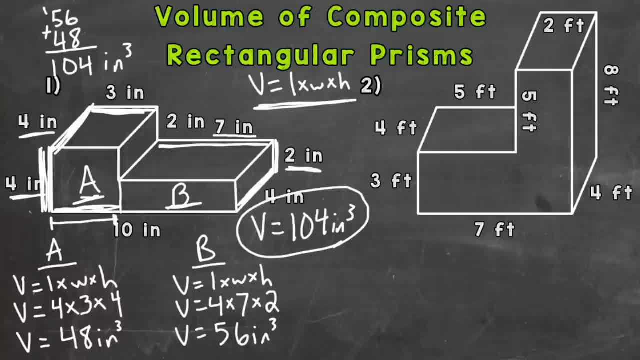 before we move to number two, I do want to mention for something. for number one, and this actually applies to all of the composite rectangular prisms, there is more than one way to cut them or split them into two rectangular prisms. so for number one, I have a left and a right I could have. 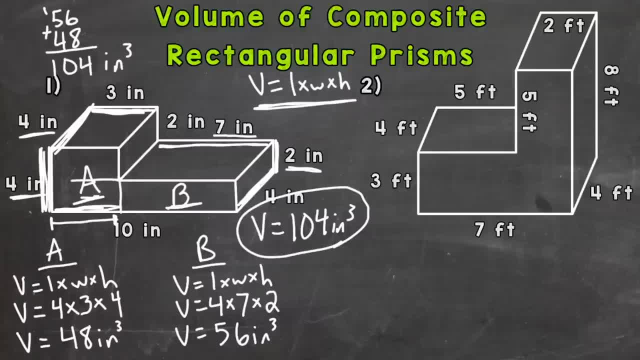 if you take a look where my letter a is, I could have cut it here, so I had a top and a bottom rectangular prism. I would have gotten to the same answer of 104. so for number two, I'm actually going to cut it. so there is a top and a bottom rectangular prism. 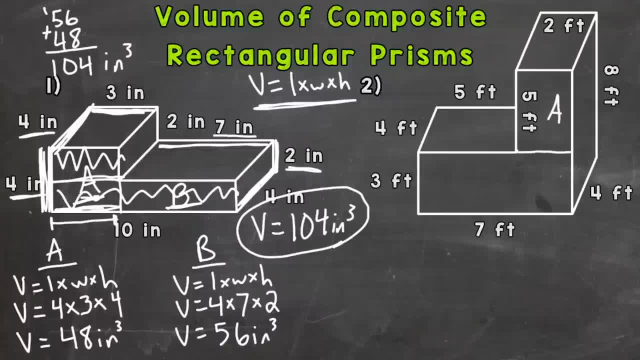 so I'm going to name the top a and the bottom B. giving them a name helps help stay organized throughout the problem. so we're going to set it up the same way as we did number one. so let's put our formulas and then it's just going to be. 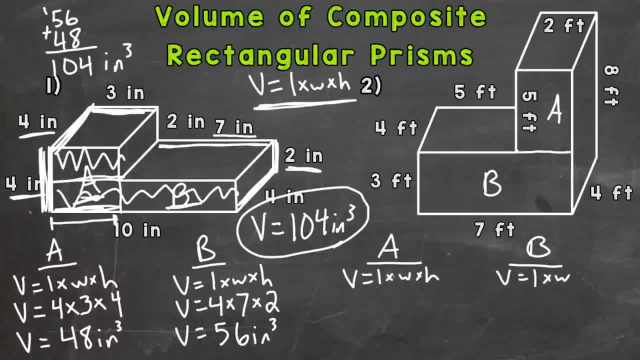 a matter of picking out the correct dimensions. So for A, we need to take a look at length. How far back does A go? Well, the whole shape actually goes. the whole rectangular prism goes back four feet, So we're going to use this four for the length A. how? 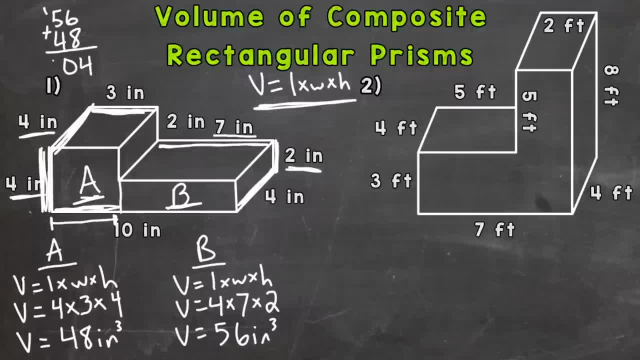 And we get to 104 cubic inches. So our answer for number 1 is 104 cubic inches. Alright, let's take a look at number 2.. Oh, actually, before we move to number 2, I do want to mention something for number 1.. 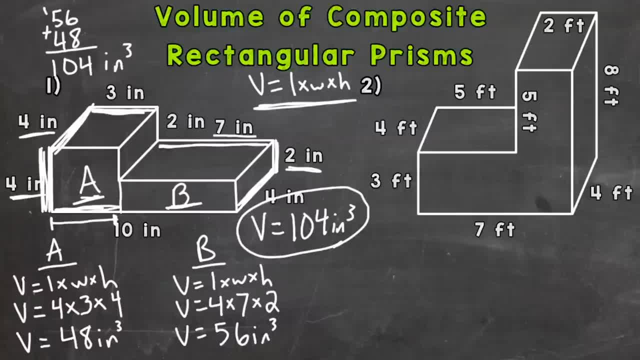 And this actually applies to all of the composite rectangular prisms. There is more than one way to cut them or split them into two rectangular prisms. So for number 1, I have a left and a right I could have. if you take a look where my letter A is, I could have cut it here. so I had a top and a bottom rectangular prism. 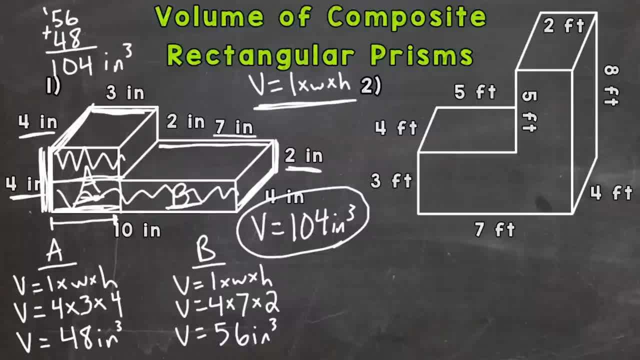 I would have gotten to the same answer of 104.. So for number 2, I'm actually going to, I'm actually going to cut it. so there is a top and a bottom rectangular prism, So I'm going to name the top A and the bottom B. 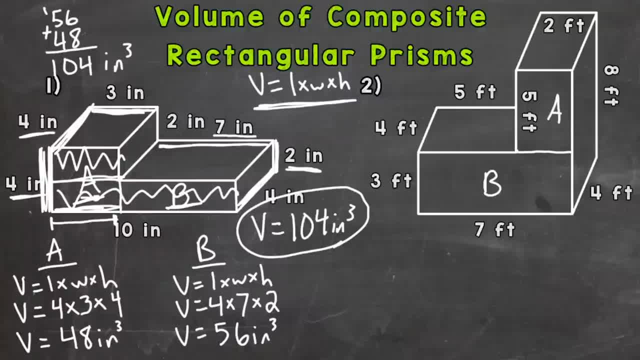 Giving them a name helps stay organized throughout the problem. So we're going to set it up the same way as we did number 1.. So let's put our formulas, And then it's just going to be a matter of picking out the correct prism. 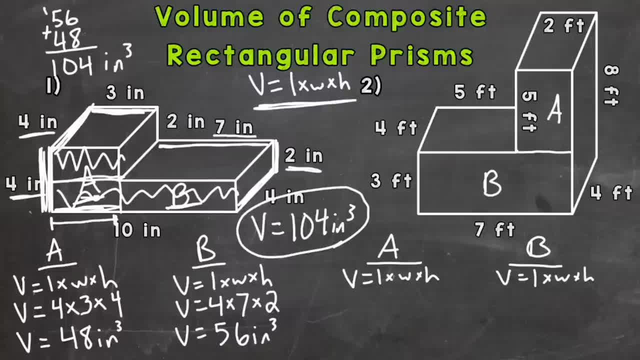 So let's put our formulas, And then it's just going to be a matter of picking out the correct prism. So let's put our formulas, And then it's just going to be a matter of picking out the correct prism. So for A, we need to take a look at length. 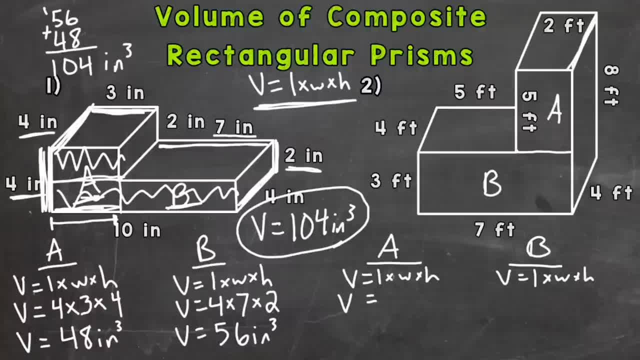 How far back does A go? Well, the whole shape actually goes. the whole rectangular prism goes back 4 feet, So we're going to use this 4 for the length. A. how wide? Well, we could look up top here and see 2 feet. 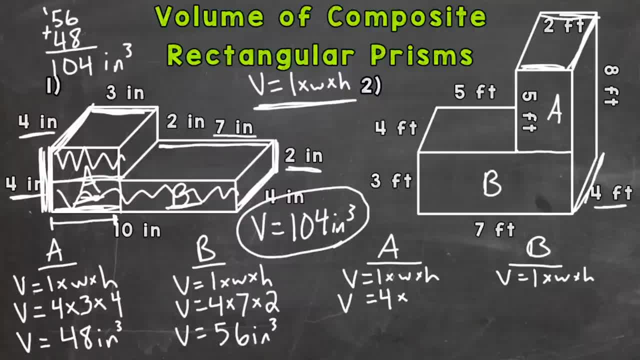 wide. Well, we can look up top here and see two feet and then the height. we don't want to use this eight over here. we don't want to use that eight because that's the whole height of A and B. We just want a, which is going to be this: 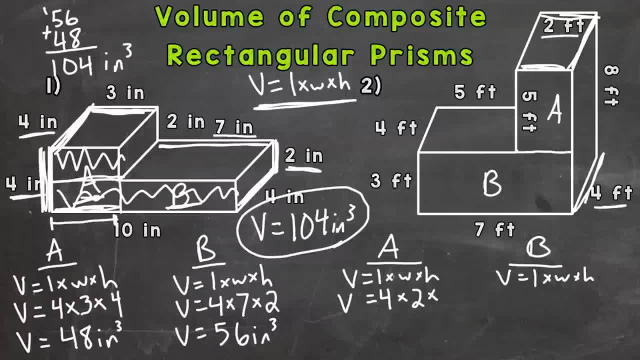 And then the height. we don't want to use this 8 over here. We don't want to use that 8 because that's the whole height of A and B. We just want A, which is going to be this 5 feet here. 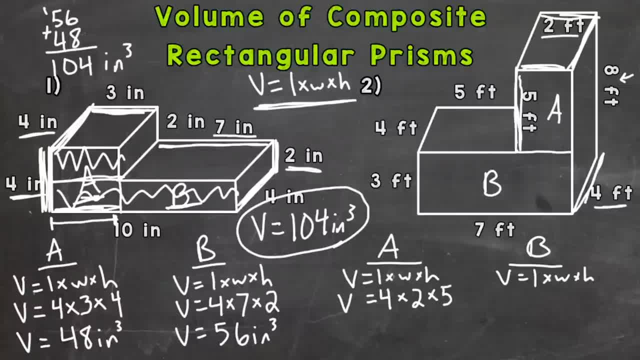 five feet here. So we get to four times two is eight times five, Great is 40 cubic feet. Now for B, the length. Well, that whole rectangular prism, or composite rectangular prism, all of it goes back four feet, which again we use this for here. 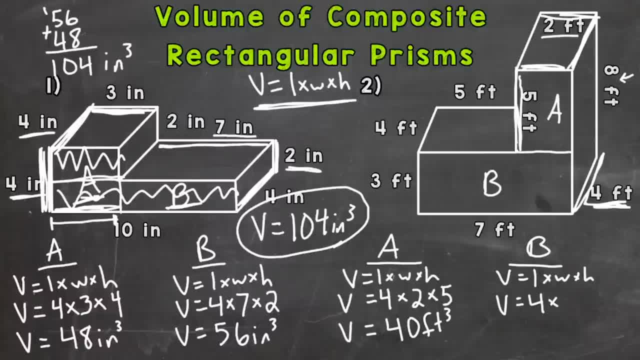 And then we need to multiply it by the width. Now B does go all the way across, So we can use this seven. Don't use this five here. That five won't be used. It doesn't go all the way across, So again we need this seven. And then times the height of. don't use the eight. 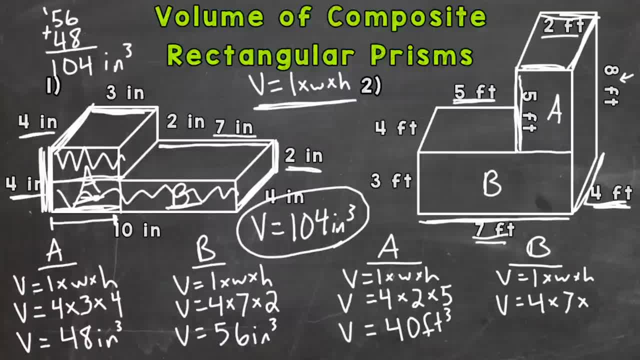 because, again, the eight is all the way up. It includes A and B. So we want right here, which is this: three feet. You do not have to use all of the numbers when you're multiplying. You do not have to use all of the numbers when you're multiplying. 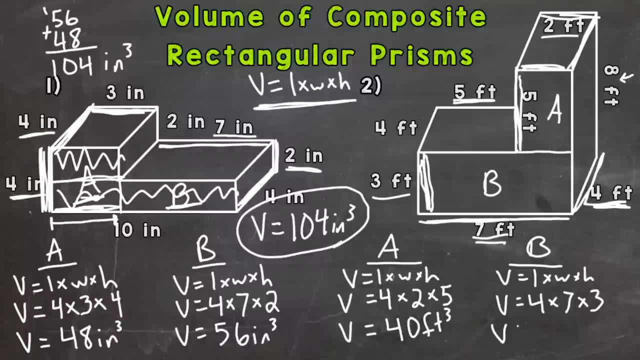 You get to these types of problems. So four times seven is 28.. And then 28 times three is 84 cubic feet. So we get to 40 plus 84, which is going to give us 124 cubic feet. So I'm going. 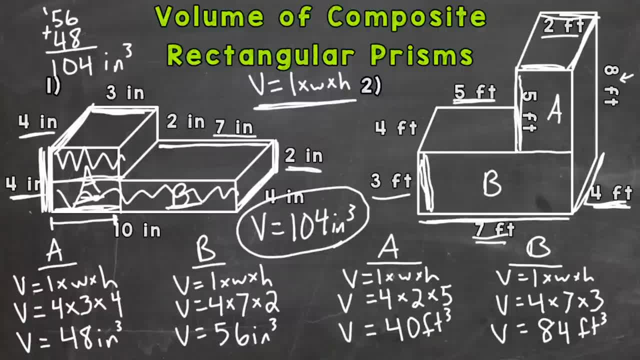 to write it inside Of our composite rectangular prism- here, because I'm running out of room. So 124 cubic feet. So there you have it. There's how to calculate the volume of composite rectangular prisms. Break your figure down into two rectangular prisms and then add those volumes together to get. 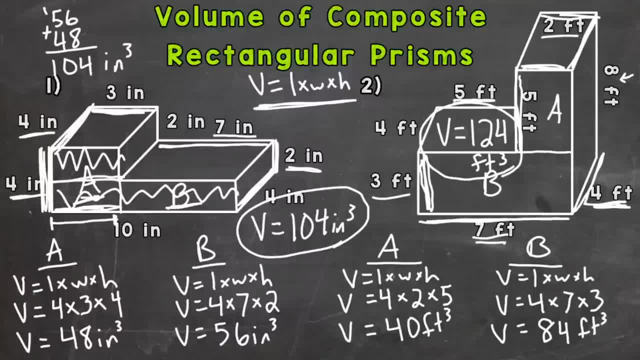 the volume of the entire figure. I hope that helped. Thanks so much for watching. Until next time, peace. 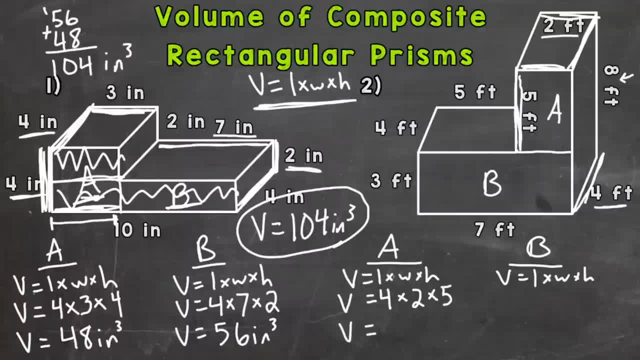 So we get to: 4 times 2 is 8 times 5 is 40 cubic feet. Now for B the length. Well, that whole rectangular prism or composite rectangular prism, all of it goes back 4 feet, Which again we use this 4 here. 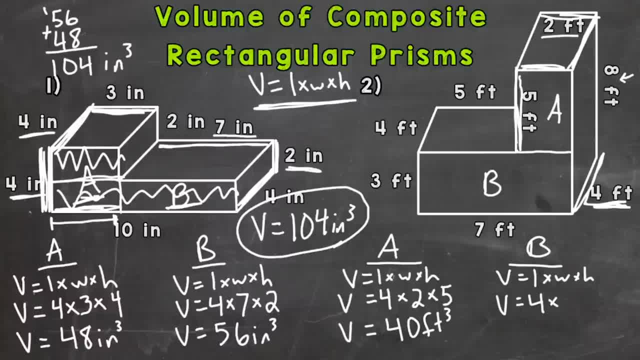 And then we need to multiply it by the width. Now B does go all the way across, So we can use this 7.. Don't use this 5 here. That 5 won't be used. It doesn't go all the way across. 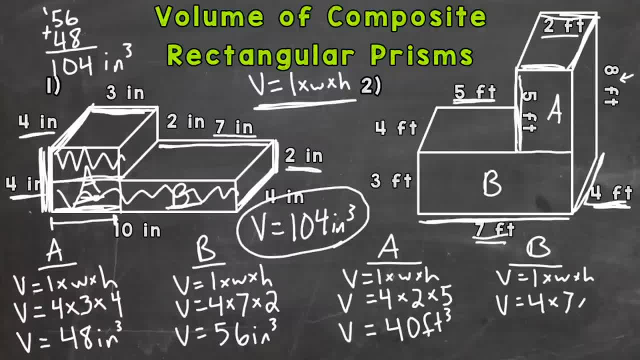 So again, we need this 7.. And then times the height of. don't use the 8. Because, again, the 8 is all the way up, It includes A and B. So we want right here, which is this, 3 feet. 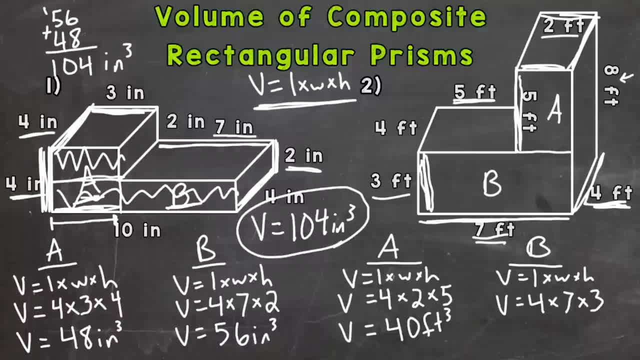 You do not have to use all of the numbers when you get to these types of problems. So 4 times 7 is 28.. And then 28 times 3 is 84 cubic feet. So we get to 40 plus 84, which is going to give us 124 cubic feet. 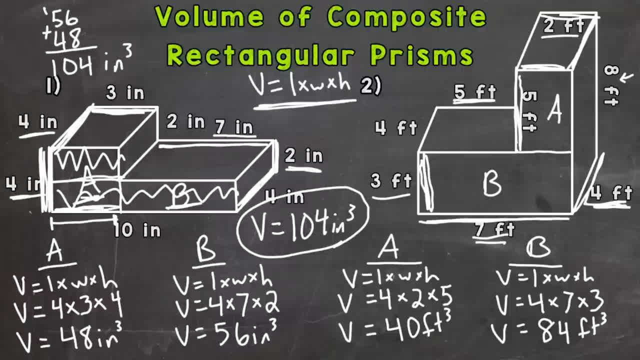 So I'm going to write it inside of our composite rectangular prism here, Because I'm running out of room. So 124. Cubic Feet. So there you have it. There's how to calculate the volume of composite rectangular prisms. 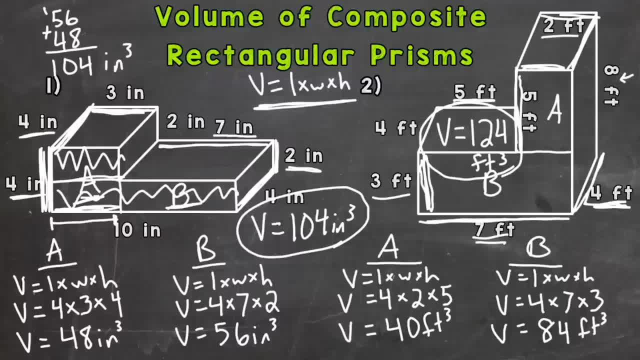 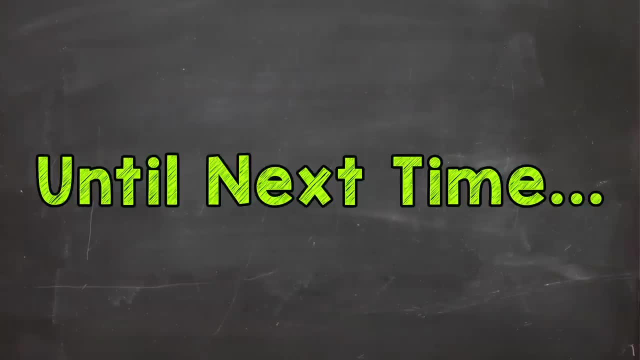 Break your figure down into two rectangular prisms And then add those volumes together to get the volume of the entire figure. Hopefully that helped. Thanks so much for watching. Until next time, Peace, Bye, bye.